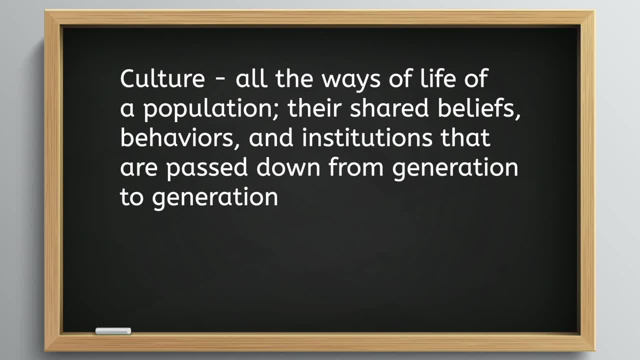 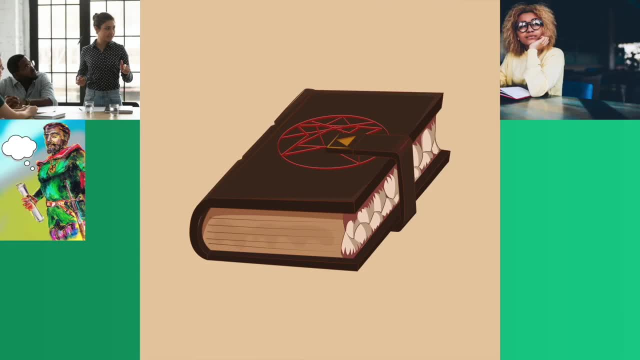 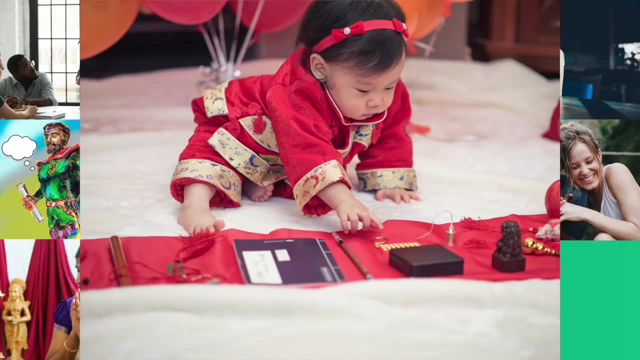 It might be simpler to think of culture as a way of life, but it's not. Let's think of it like this: Practically anything that humans say, do think, discuss, write, read, eat, protest, love, pray, to meditate upon, turn away from or live up to can be. 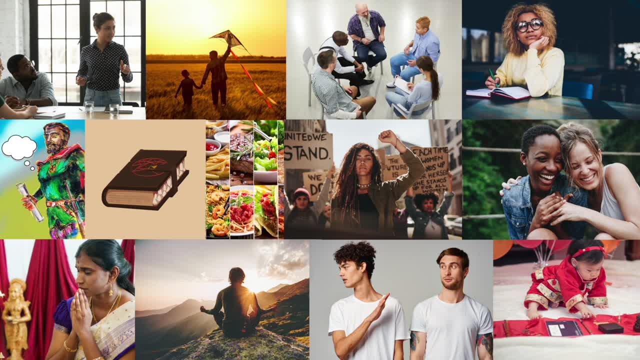 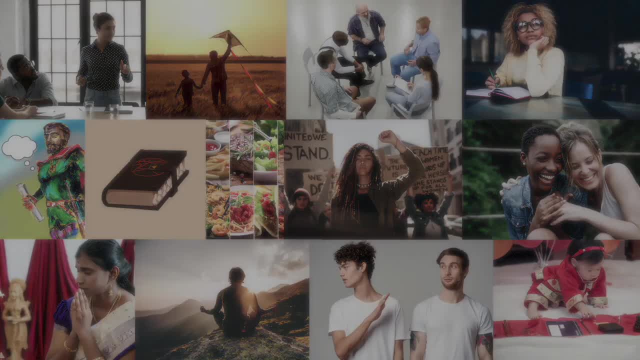 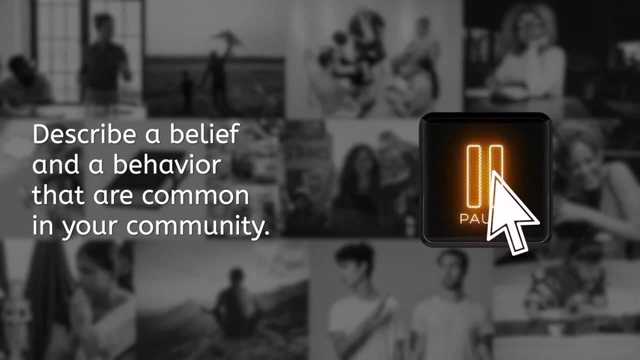 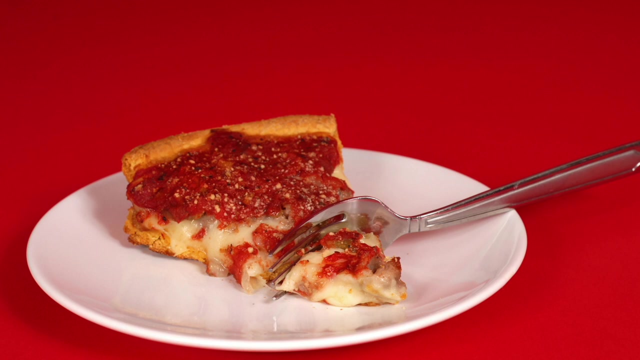 considered a part of culture, and that just scratches the surface. Let's begin our journey to learn about culture by describing a few of our own traits In your lesson guide. describe a belief and a behavior that are common in your community. Maybe you said that in your town people believe that pizza should be deep dish and they eat it with a fork. 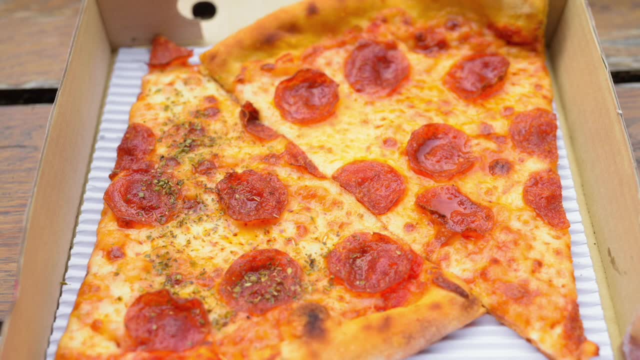 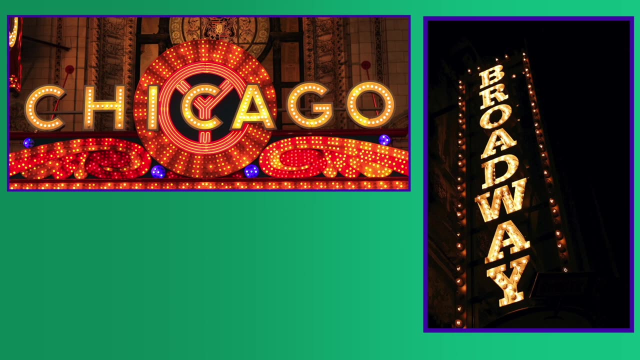 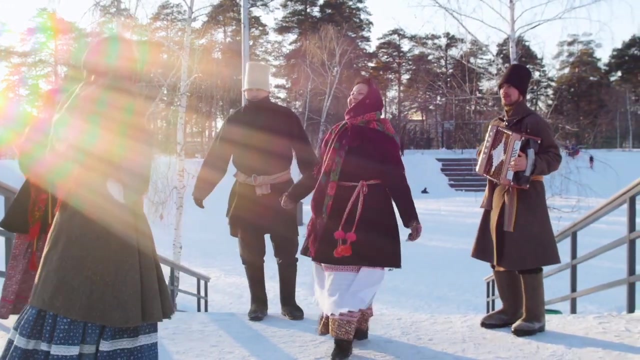 Or maybe because of where you're from, that sounds horrifying. The things we could look at even between two cities like New York and Chicago could take us years to comb through. We just don't have time to do a deep dive on every cultural group in every country this year. 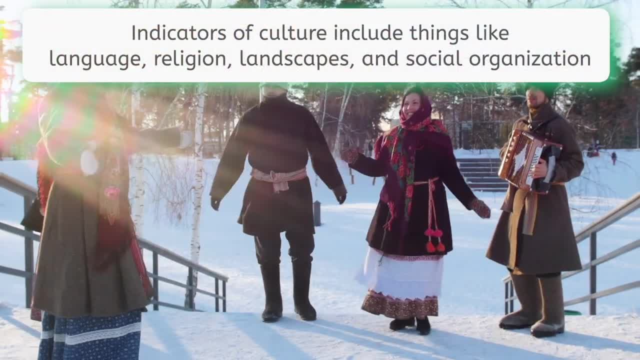 But we can talk about culture in every country this year. But we can talk about culture in every country this year, But we can talk about culture in every country this year And we've got a few key indicators of culture that will help us understand the people we will encounter in our trip around the world. 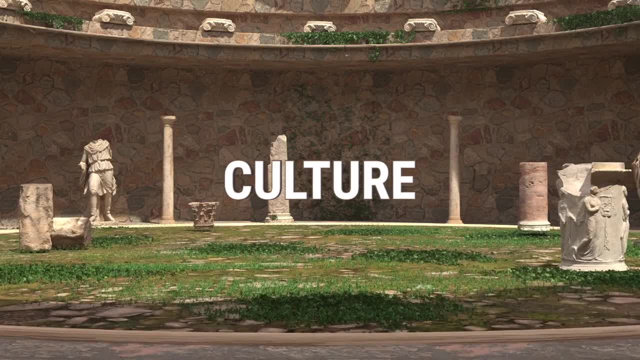 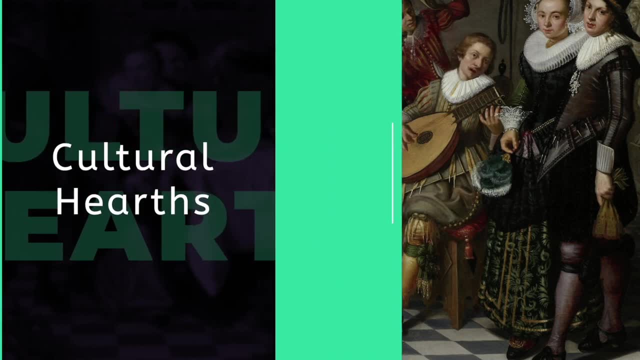 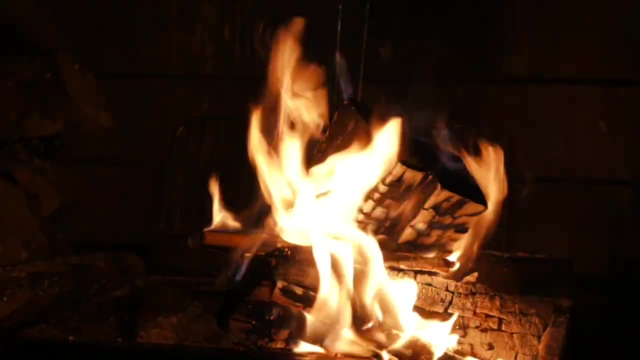 Let's start by taking it back to our humble beginnings, the cultural hearth. You may be somewhat familiar with the word hearth through a commonly used phrase like hearth and home. Most people assume that a hearth is a fireplace or an oven. 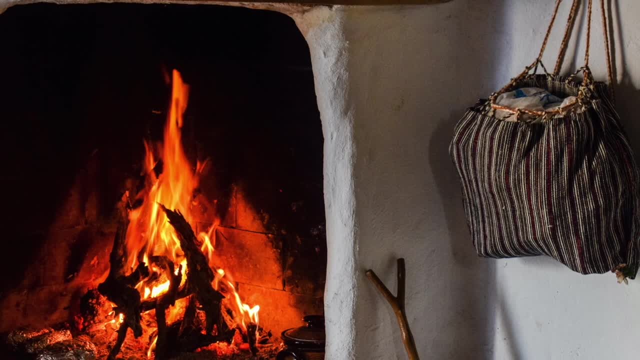 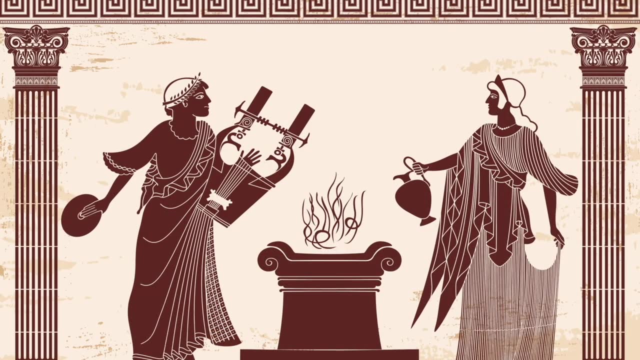 But for many peoples, like the ancient Greeks, a hearth was considered the center of the home, the focus of all family activity. This was where kids were taught and where stories were told. A cultural hearth is where people gather and express themselves. 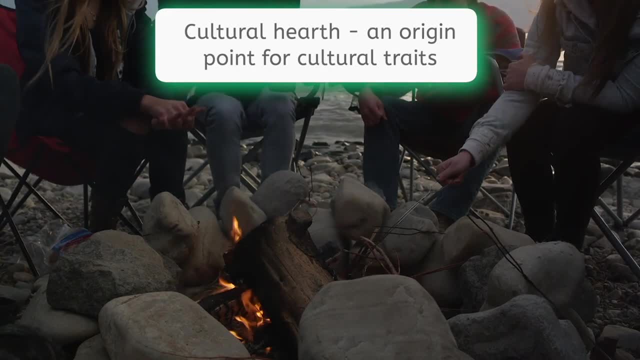 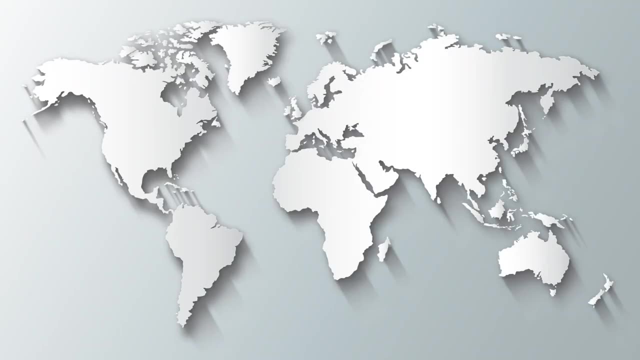 A place where their culture lives and breathes freely, A point from which it spreads, much like warmth spreads from a fire. Most of the earliest cultural hearths are places where agriculture first developed. They are widely recognized as river valleys along the Nile. 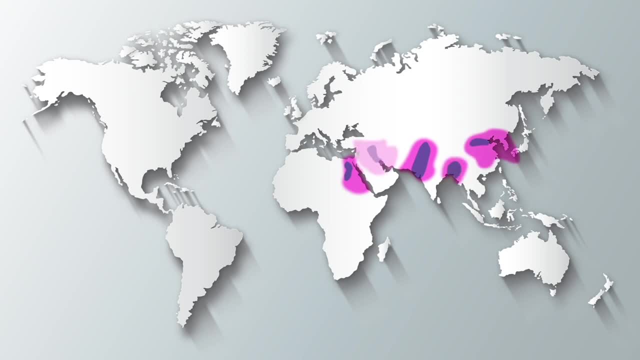 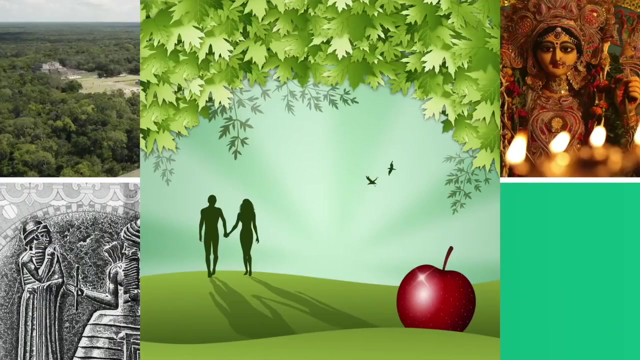 Indus, Yellow Ganges, the Tigris and Euphrates rivers, Central and South America and West Africa. Within each of these areas, civilizations emerged. They developed language, religion, laws, skills and origin stories which still influence us today. 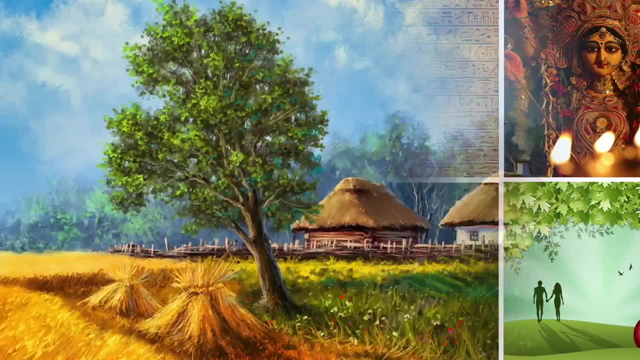 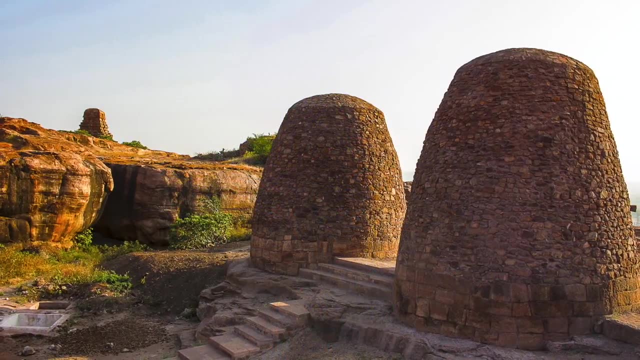 So what drove the development of these hearths? As larger groups of people lived together, they standardized certain things like farming to feed everyone. Standard rules and systems allowed humans to live and work together, and these rules were passed on to later generations. 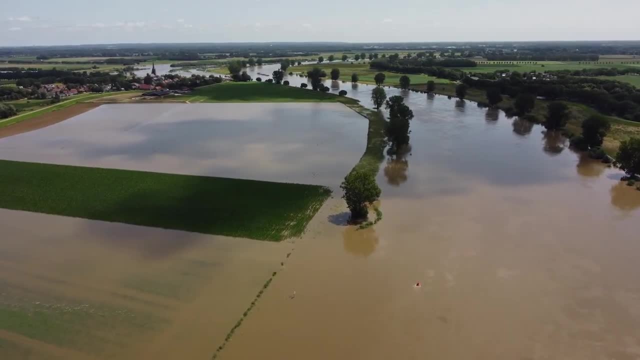 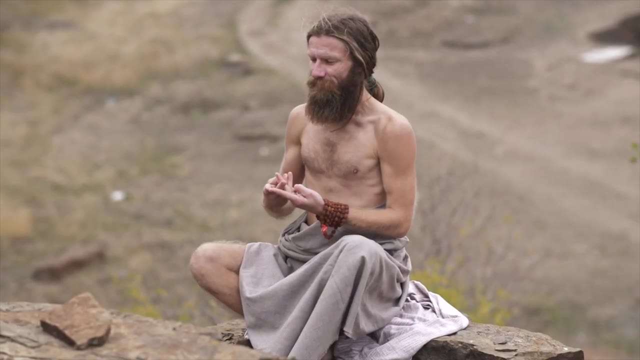 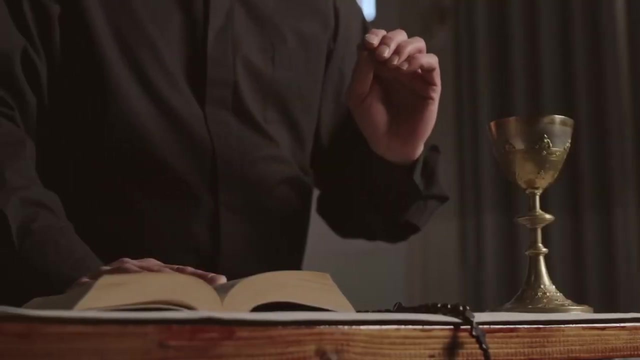 As settlements grew, they encountered new problems like the effects of floods. They studied storms and seasons and marked the passage of time. Religious practices, philosophical ideas and methods of measuring goods and services came next. As time went on, these beliefs, behaviors and institutions were spread to new peoples. 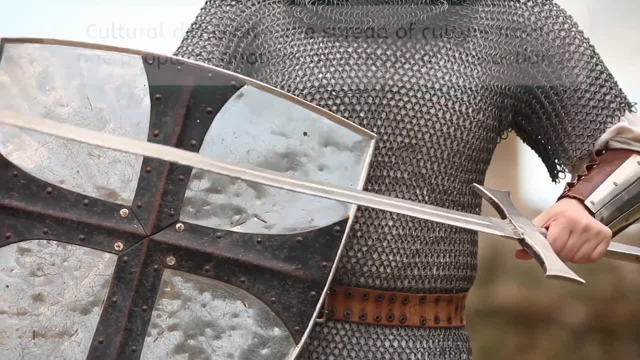 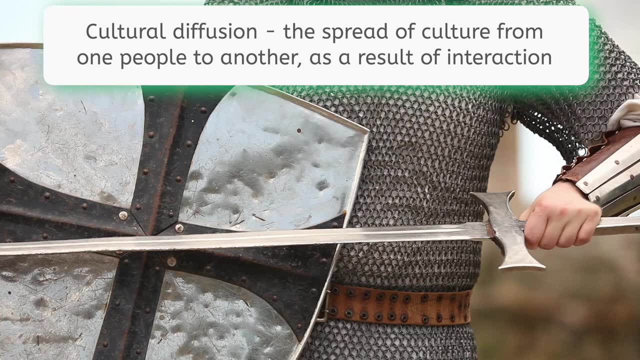 through travel and through the use of technology, They were able to build new systems to travel, trade and war in a process called cultural diffusion. Show what you know about hearths and diffusion in your lesson guide. In your own words, what is a cultural hearth? 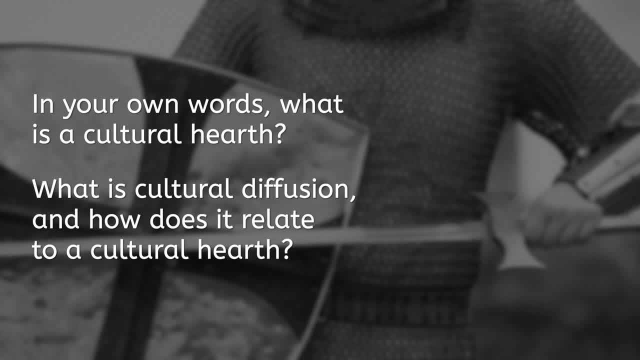 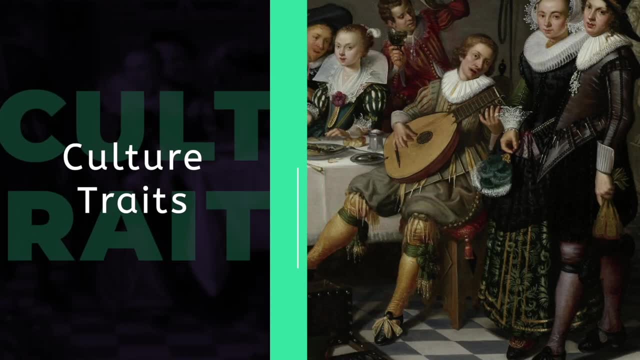 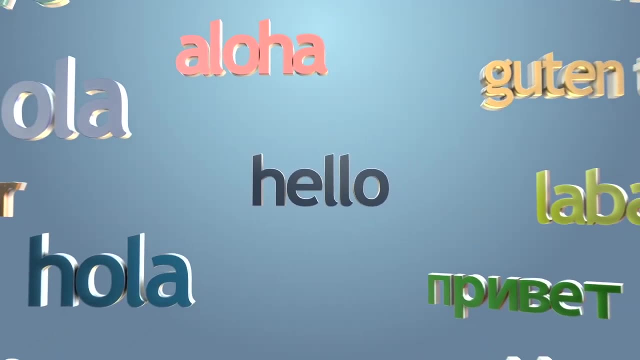 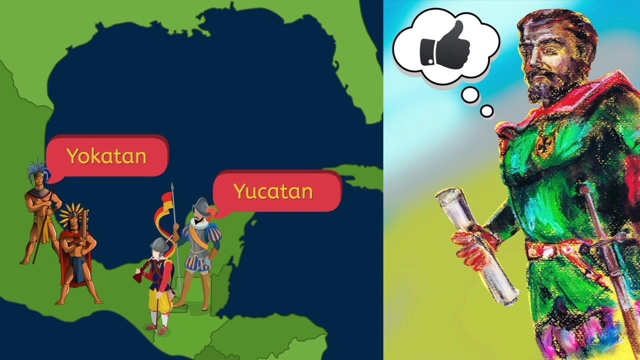 What is cultural diffusion and how does it relate to a cultural hearth? Cultural diffusion and cultural hearth. One of the most important cultural features that a geographer can look for is language. Without knowing the local dialect, de Córdova ended up naming an entire peninsula- something. 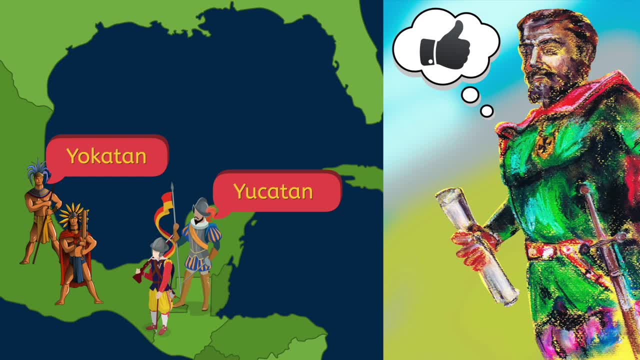 that may have meant I don't understand you. Not knowing a language isn't just a lack of understanding of the literal meaning of words. it's also a matter of context. People learning English as a second language often struggle with common phrases like break. 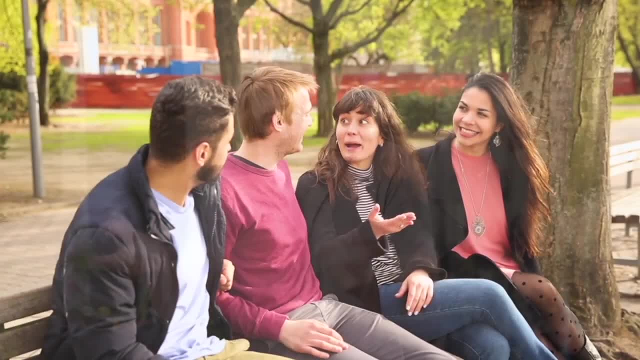 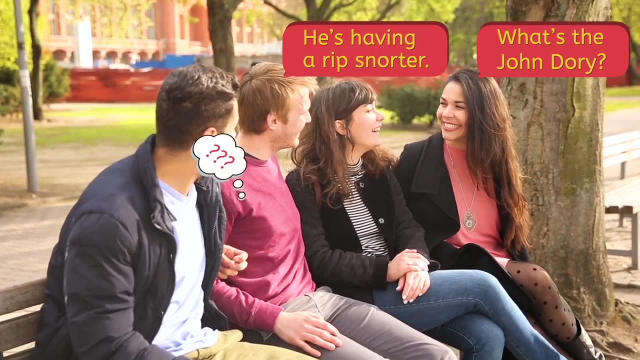 a leg or a piece of cake. But in the same way, American English speakers wouldn't understand an Australian phrase like what's a John Dory? or he's having a rip snorter. Regional differences often reflect the experience of living in a particular place. 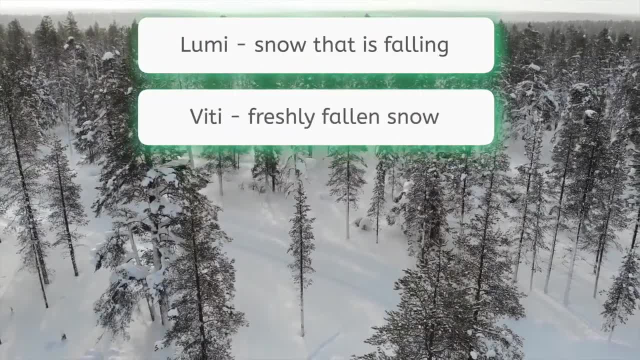 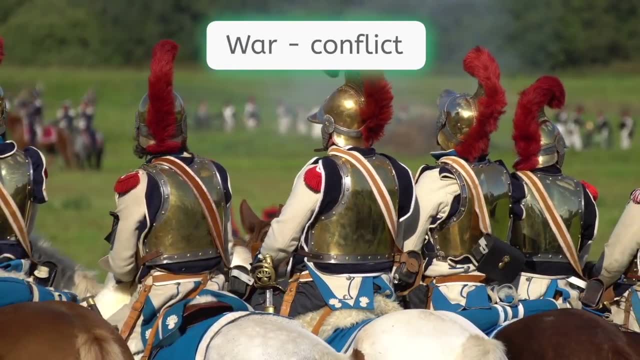 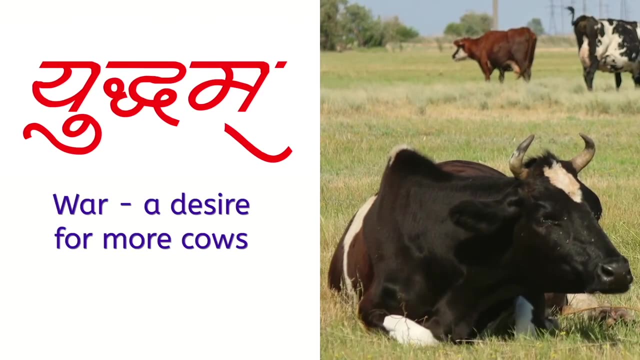 In Finnish there are over 40 words for snow, and each has a distinct meaning. Language can also reflect a powerful connection to the past. In most languages the word for war means conflict, but in Sanskrit it translates to a desire for more cows, because it's from a time in which most people were herders and 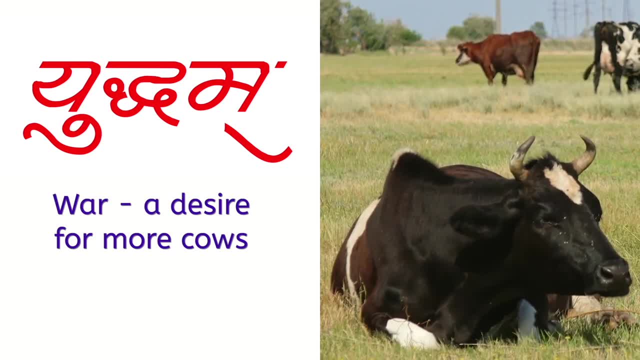 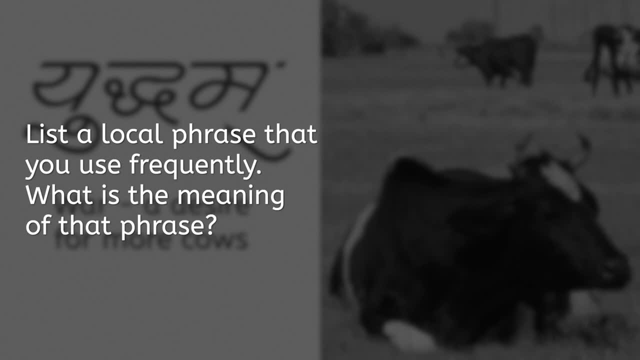 that's what they fought over. Let's reflect on the context embedded in our words. List, a local phrase that you use frequently. What is the meaning of that phrase? Maybe you said that asking someone to ballpark? it means to estimate an amount of something. 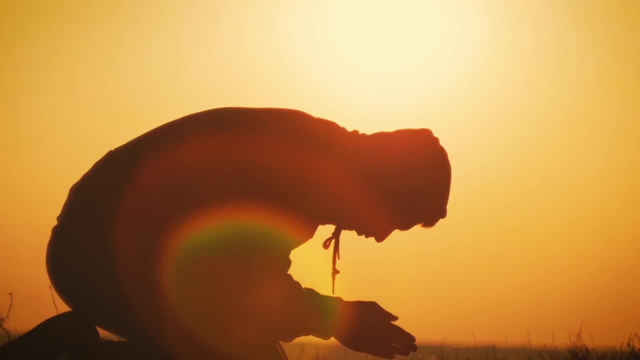 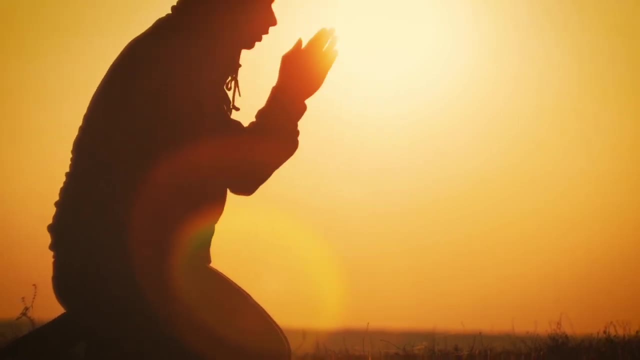 Other cultural indicators are the ideas of faith. It's important to understand the meaning of the word. It's important to understand the meaning of faith and religion. What happens to people after they die and how should we treat others are questions that every population has its own answers for. 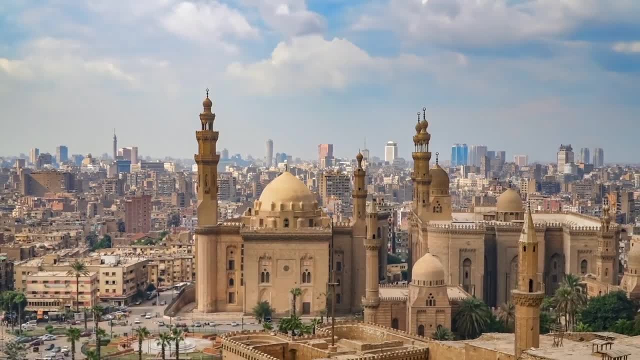 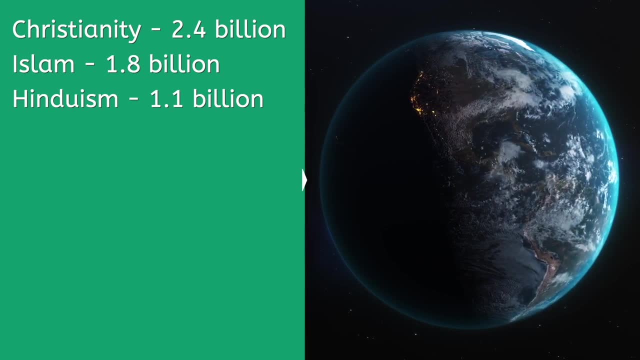 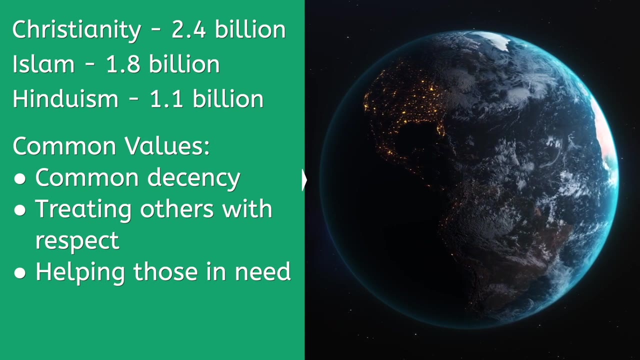 Answers which, like language, derive from living in a particular society. 5.3 of the world's 8 billion people are followers of either Christianity, Islam or Hinduism, But people of many faiths hold similar values of common decency, treating others with respect. 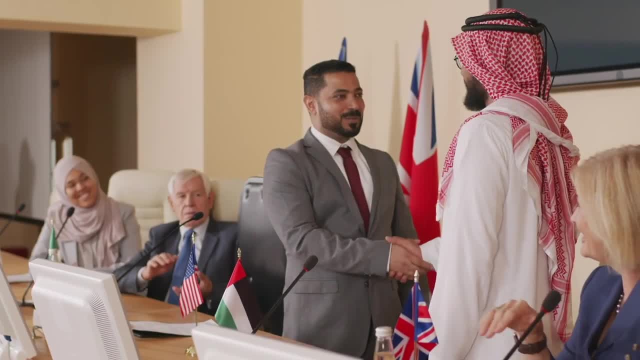 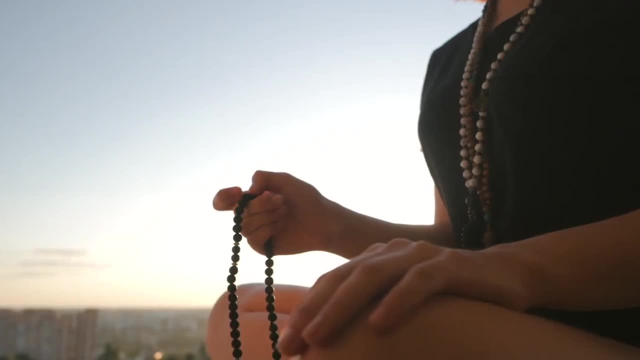 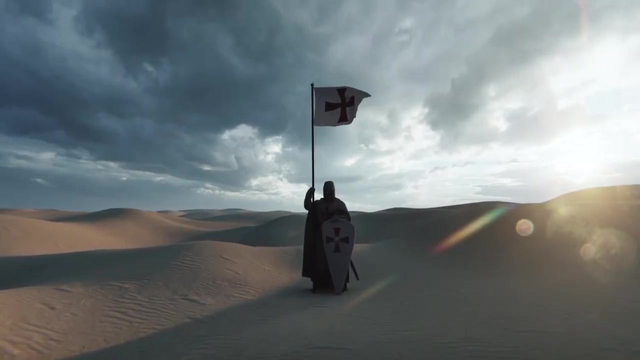 and helping those in need. So even people of different religious traditions can have somewhat of a cultural understanding through these teachings. Religion can be a powerful motivator for providing aid to communities throughout the world, but can also provide an unyielding ideology leading to acts of violence. 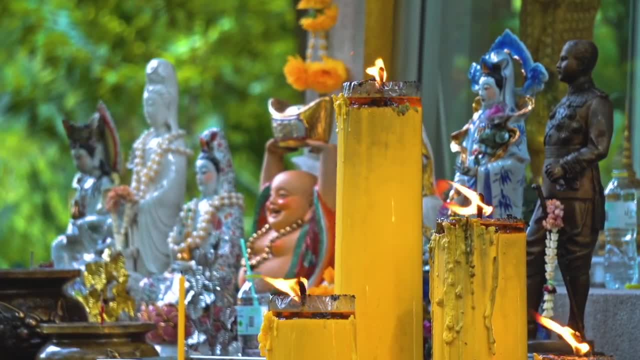 As we look at followers of major religions around the world. in later units pay attention to the powerful influence of faith and religious practice in place and space. 6.3 of the world's 8 billion people are followers of either Christianity, Islam or Hinduism. 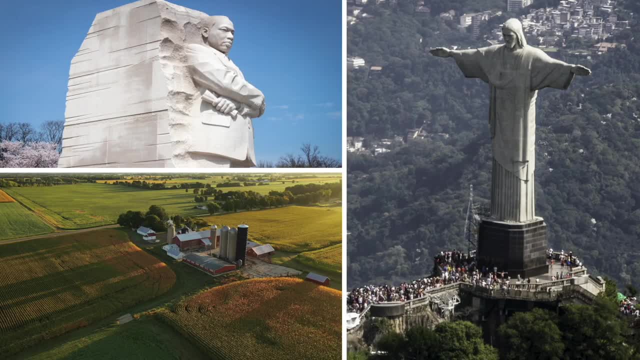 7.3 of the world's 8 billion people are followers of either Christianity, Islam or Hinduism. 8.3 of the world's 8 billion people are followers of either Christianity, Islam or Hinduism. 9.3 of the world's 8 billion people are followers of either Christianity, Islam or Hinduism. 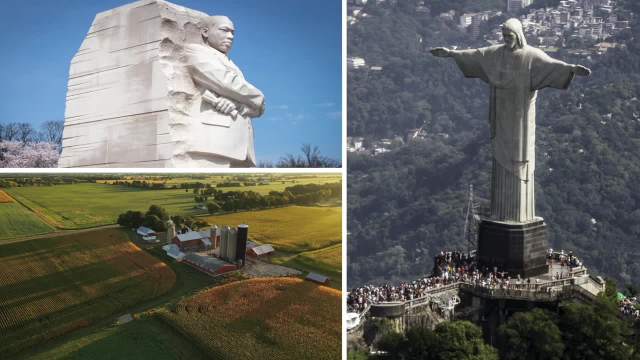 This is why a cultural chance is so important in our society. Once you've understood your cultural chance, you will take advantage of it at a higher level of spirituality. By looking at the following images, you will understand your cultural chance at being a part of the culture of your country. 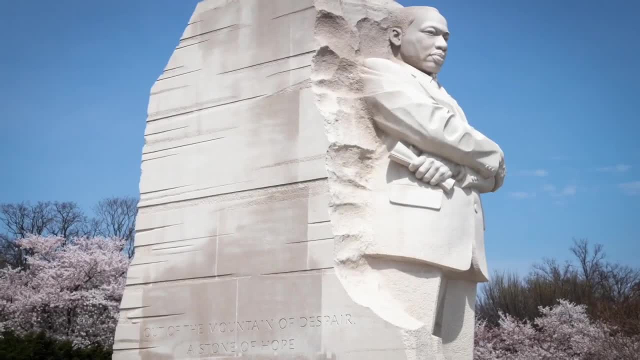 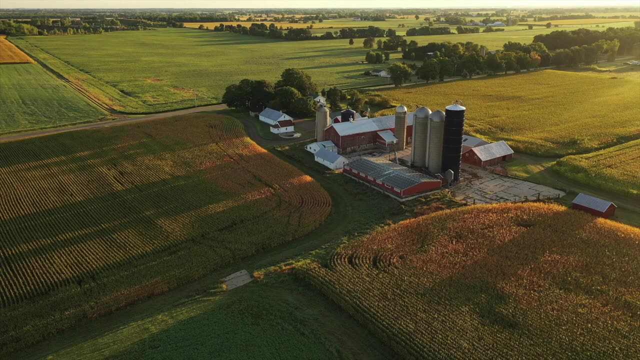 The educator of culture can be seen in the landscape. What culturally important concept is on display in these images? Whether as a tribute to an important icon, monument of faith or piece of land sewn with crops, all convey a sense of cultural landscape in their usage. 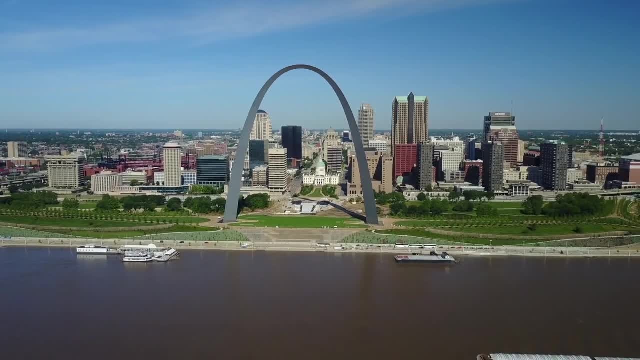 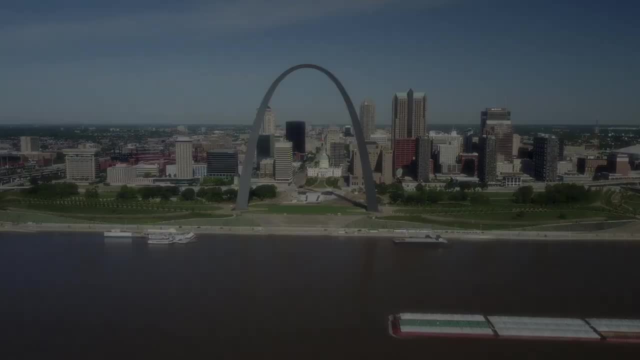 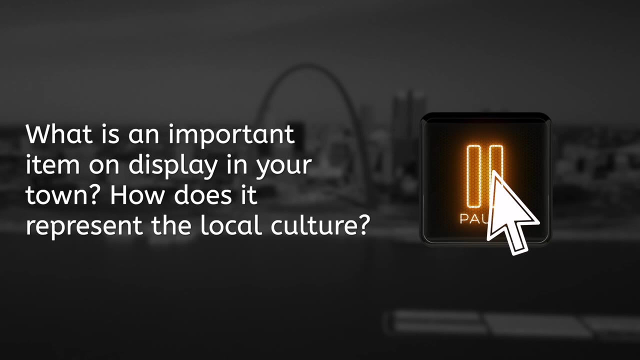 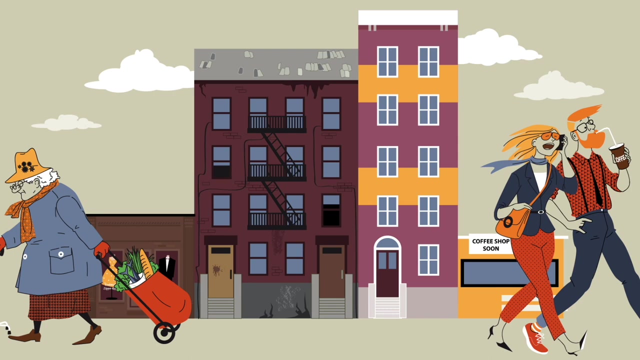 When considering cultural landscapes, the geographer should always ask what culturally important idea is being conveyed. What about your cultural vision, community? Pause the video here and name an important item on display in your town. How does it represent the local culture? Social organization can also help the geographer to learn about latent